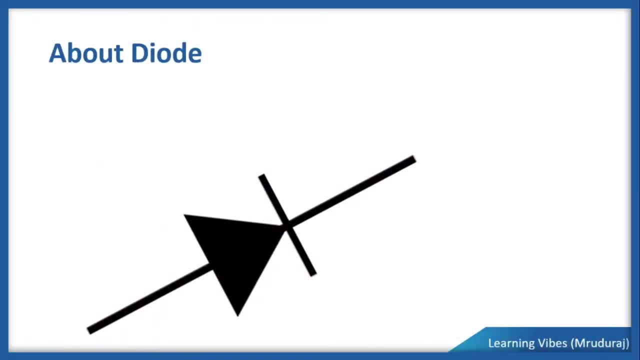 Hey everyone, I hope you all are fine. In this session, we all are going to learn how to identify the terminals of diode. The next thing we are going to discuss in the same video, that is how to connect this diode in forward and reverse bias condition. 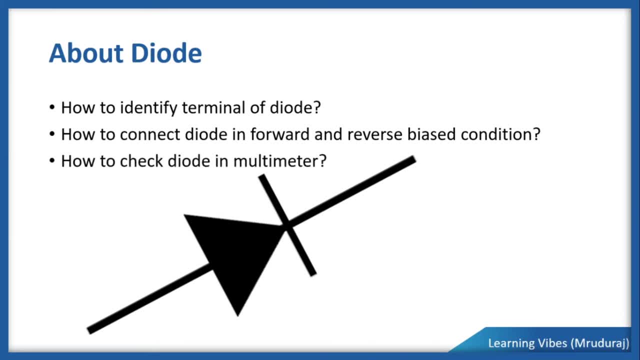 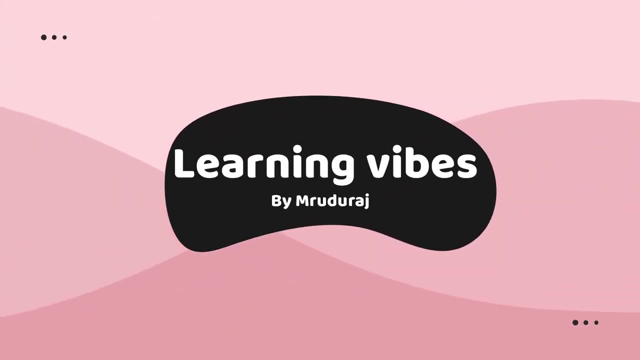 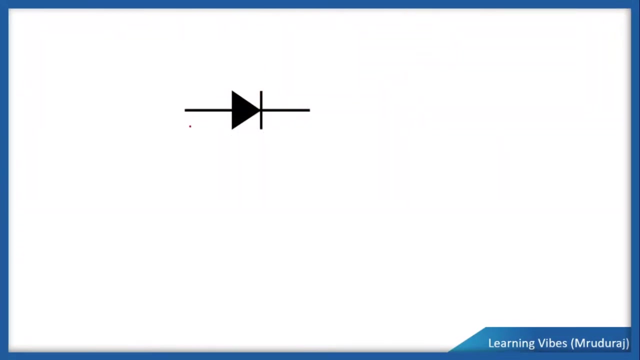 And the third thing that we are going to discuss is how to check the diode in multimeter. So these three important things we are going to learn in this video. So, without wasting time, let's begin with the first thing. This is the symbol of diode. There are two terminals in this symbol. 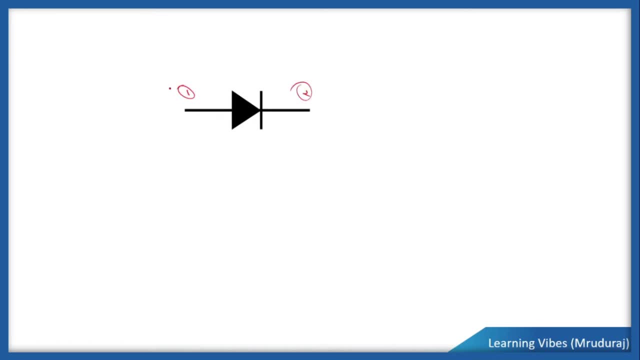 This is terminal number 1 and the terminal number 2.. The terminal number 1 is known as anode, The terminal number 2 is known as cathode And you all are aware. with this, You are not here to understand this thing. 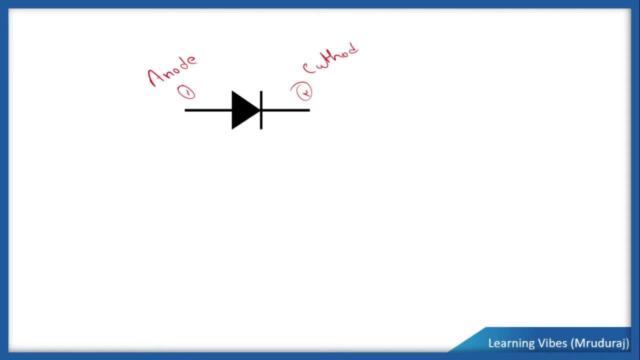 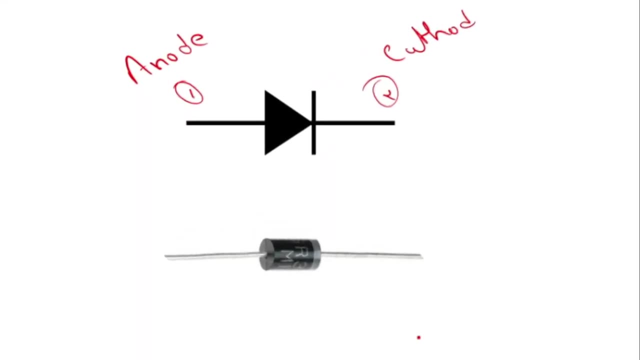 You are here to know how to identify terminal of diode, of a real diode. So this is the real diode. When you see a real diode, the diode looks like this, And now let's understand how to identify which one is anode and which one is cathode in real diode. 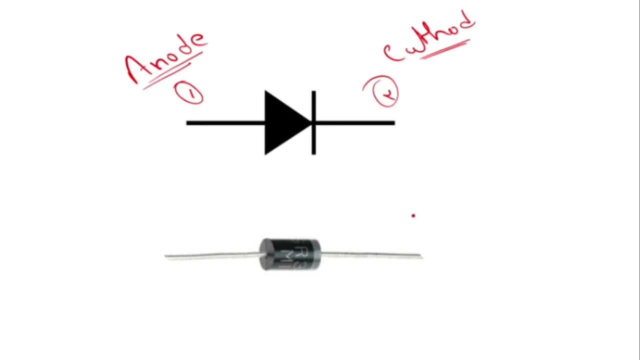 This silver line indicates the cathode. So whenever you see the real diode, this silver lining represents the cathode. In this condition, this silver line is the cathode And this silver lining is on this side. So this terminal of diode is cathode terminal. 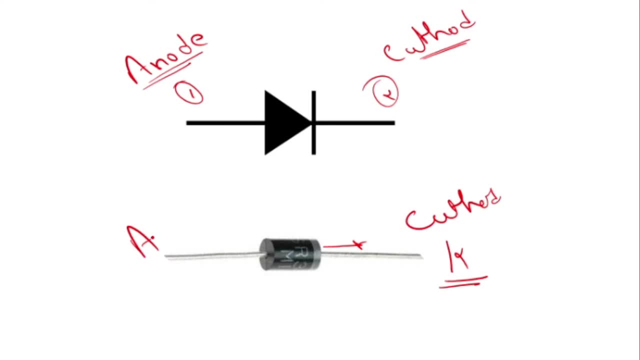 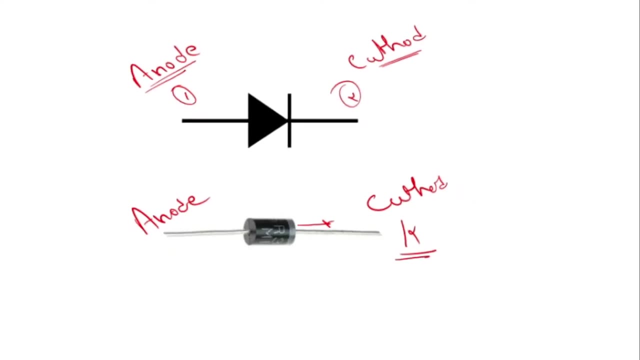 Over here there is no silver line, That means this terminal is anode terminal, And this is one of the easiest method to identify the terminals of diodes. So wherever you find the silver line, that terminal of the diode is known as the cathode terminal. 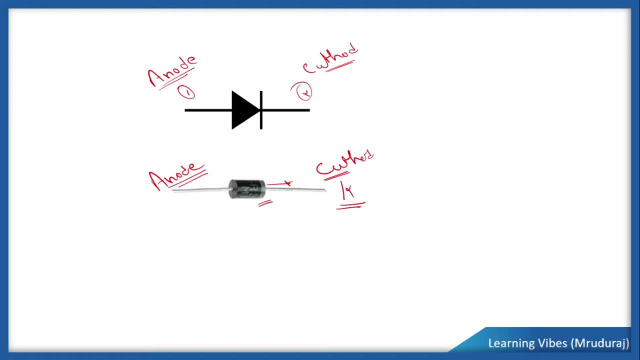 And when there is no silver line, that terminal of diode is known as the anode terminal. Basically, the anode terminal is the positive terminal of the diode and the cathode terminal is the negative terminal of the diode. Why it is so? Because it is constructed of p-type material, p-type semiconductor material, and it is constructed of n-type semiconductor material. 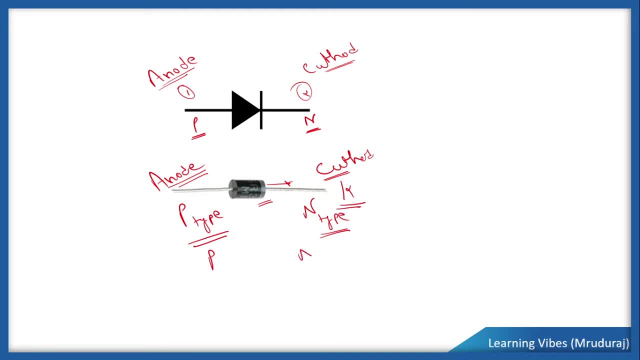 So the anode is known as the positive and the cathode is known as the negative. Simply, it is the p-type or n-type. But to understand this we need to understand the anode terminal. To understand I am representing as positive and negative. 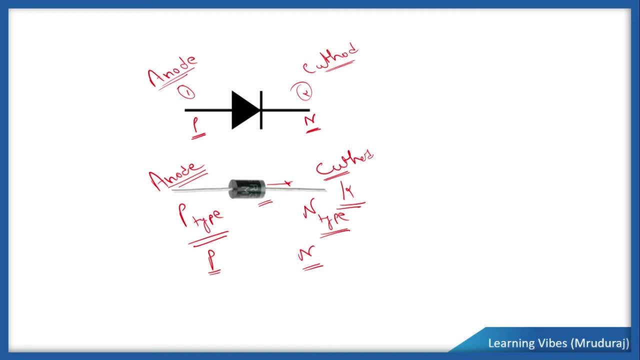 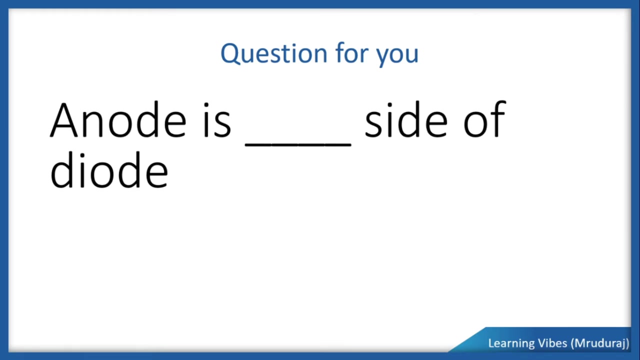 So p-type and n-type. Now we are going to learn how to connect this diode in forward bias as well as in reverse bias condition, So let's move to that. Before moving ahead, there is a small question for you, And the question is: anode, is which side of the diode, p or n? 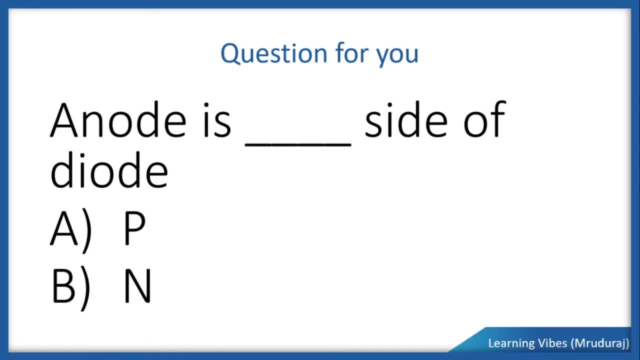 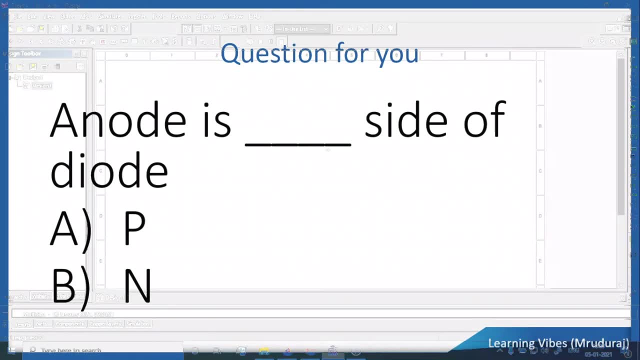 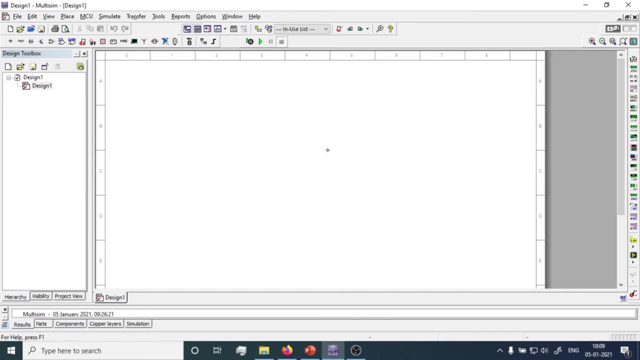 Just think quickly and answer me this question. Answer me this question in comment section quickly, Right, What is the right answer? And then we will move ahead. This thing we are going to learn with the help of simulation tool. First of all, we will prepare the forward bias circuit of the diode. 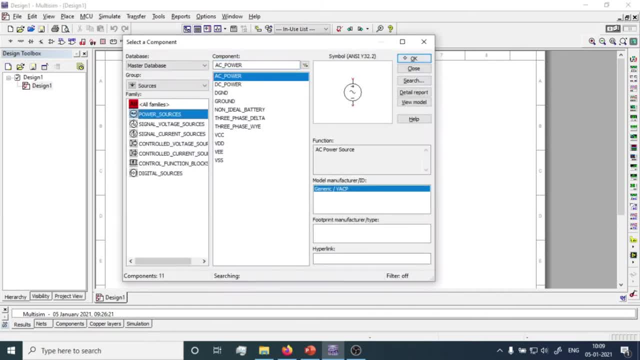 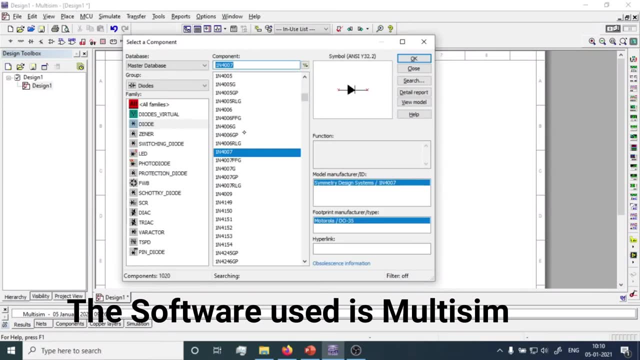 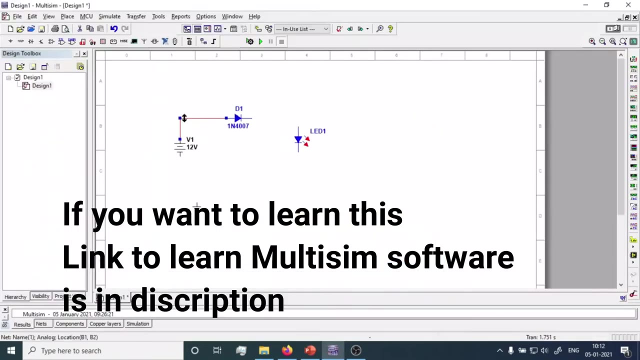 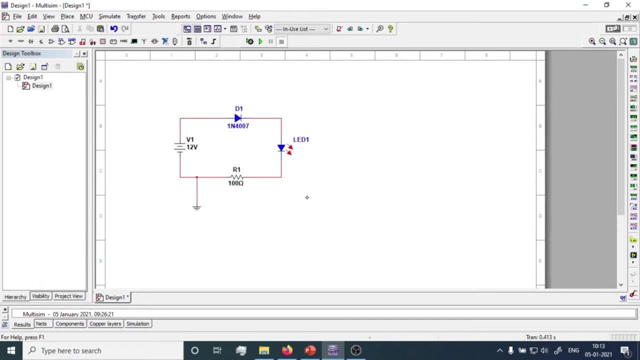 For that we will use several components. First of all we will prepare the forward bias circuit of the diode. Okay So, circuit of diode forward bias connection is ready. How the diode is connected in forward bias, This is the positive terminal of battery. 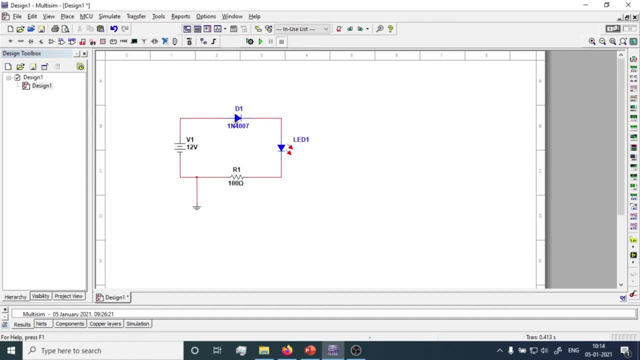 The positive of battery is connected with the positive of diode And this is the negative terminal of battery. So the negative terminal of battery is connected with the negative side of the diode. So p-side of the diode is connected with the positive of battery, whereas n-side of the diode is connected with the negative of the battery. 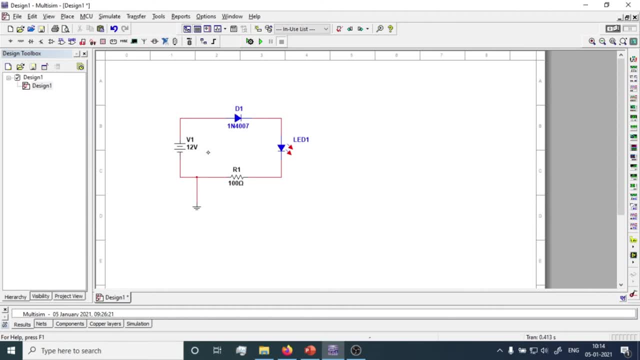 So this is the forward bias condition of the diode. Now let's play the simulation. This is the light emitting diode. If it keeps on red, that means the diode is in forward bias condition and it is conducting. So let's run the simulation. 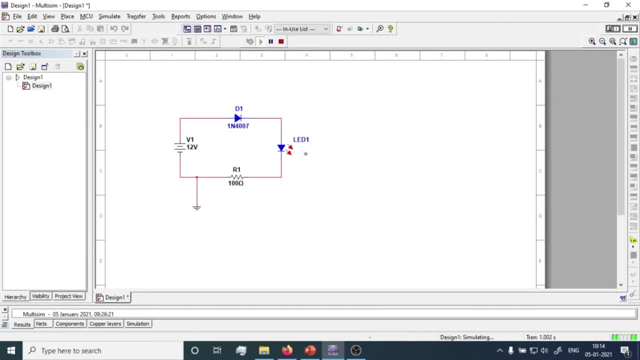 And we can see that the red line is still on Right. What we will do now? We will stop the simulation, We will select everything, We will copy and we will paste everything over here. Now we want to connect this diode in reverse bias condition. 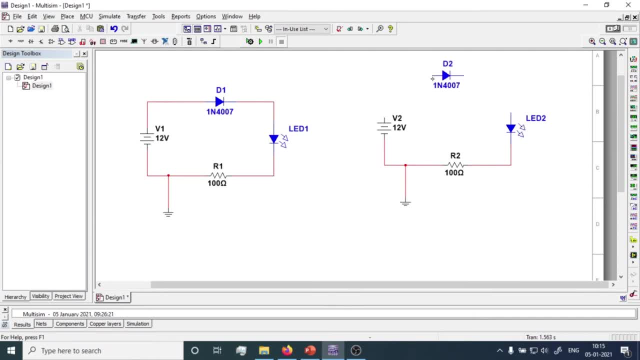 So we will remove it. Control X, Control V again, Press Control R, Control plus R two times So it will change its direction And now again connect this diode. So in this condition the positive of battery is connected to the n-side of the diode. 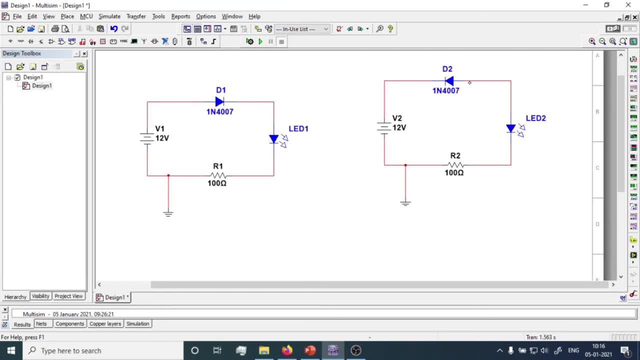 And negative of the battery is connected to the p-side of diode And this is known as the reverse bias condition And this is known as the forward bias condition of the diode. So now what we will do Again, we will run the simulation and we will observe that in forward bias condition, diode will conduct. 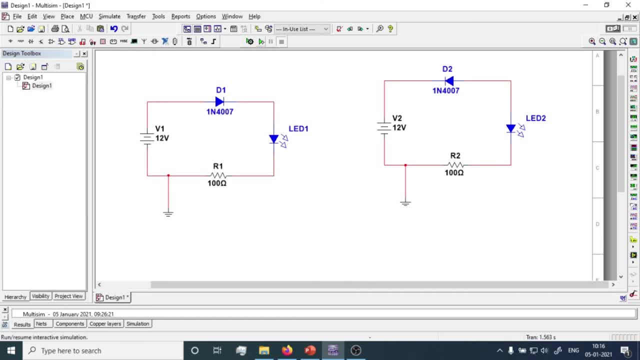 And in reverse bias condition diode will not conduct. So let's run. You can observe that when the diode is connected in forward bias, the LED is turned on, And from here you can observe that when the diode is connected in reverse bias condition, this LED will not function. 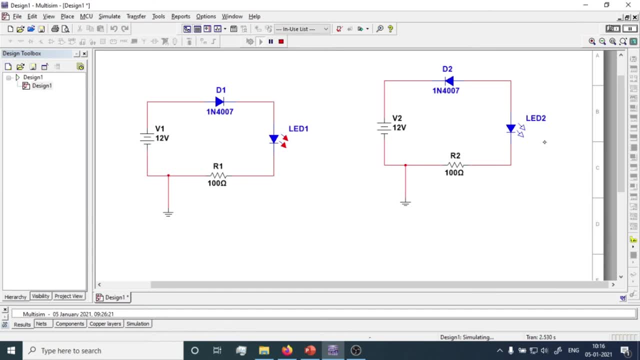 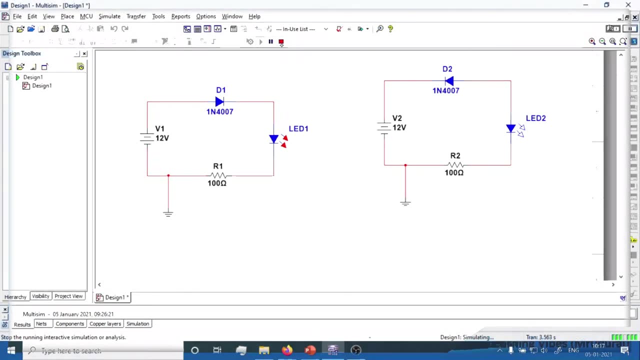 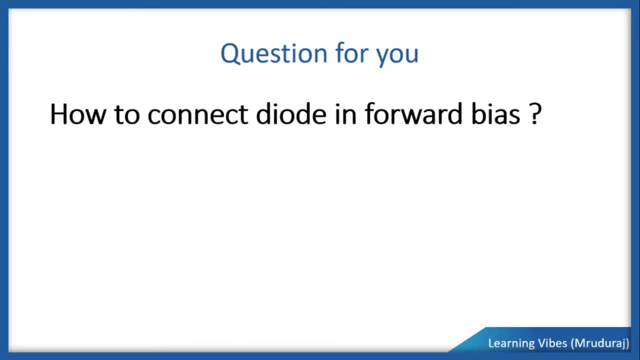 Right. So this is how you can learn how to connect diode in forward bias as well as in reverse bias condition. Now let's move for the next topic. Before moving ahead, there is a quick question for you, And the question is how to connect diode in forward bias condition. 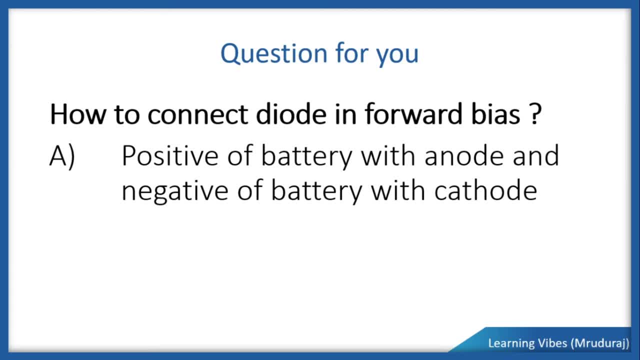 A. Positive of battery with anode and negative of battery with cathode. B- Negative of battery with anode and negative of battery with cathode. A- Positive of battery with anode and positive of battery with cathode? Answer me this question quickly in comment section below. 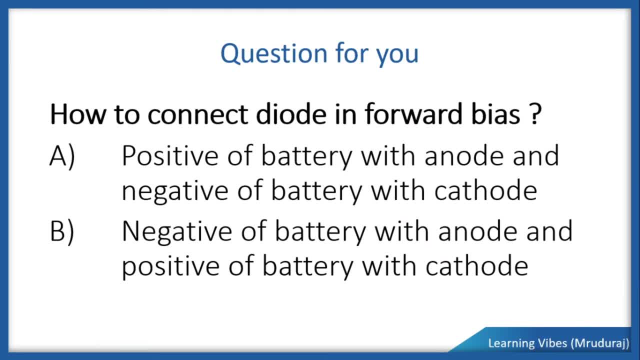 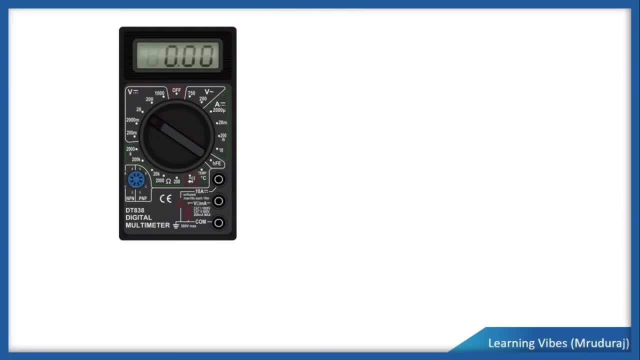 What do you think that? how to connect the diode in forward bias condition. If you have understand it properly, answer me in comment section. Now I am going to tell you how to check the diode with multimeter. I have prepared the same video for this thing.